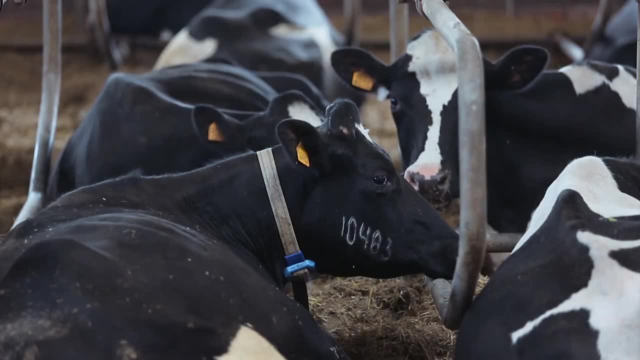 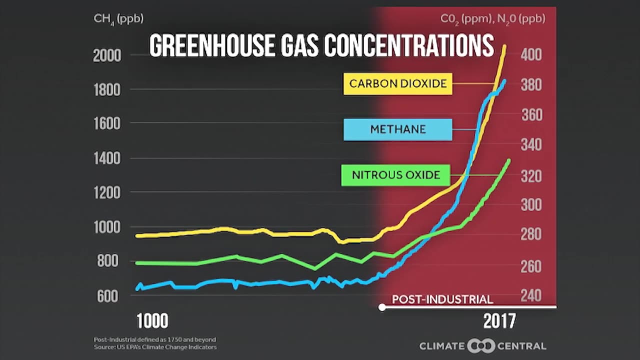 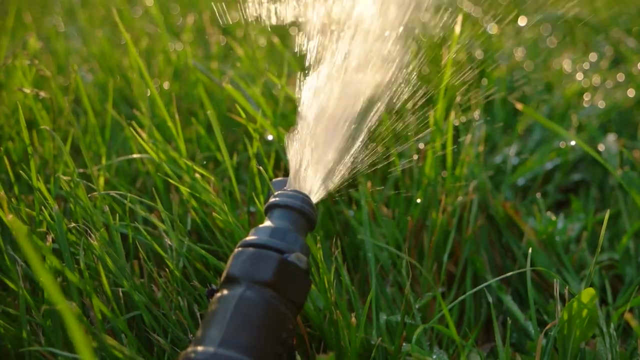 Livestock produce methane as they digest their food. Then their manure produces even more methane as it decomposes. Methane is 30 times more potent than carbon dioxide as a heat-trapping gas for the planet. That means meat production contributes to climate change, which in turn contributes to the world's onshore. 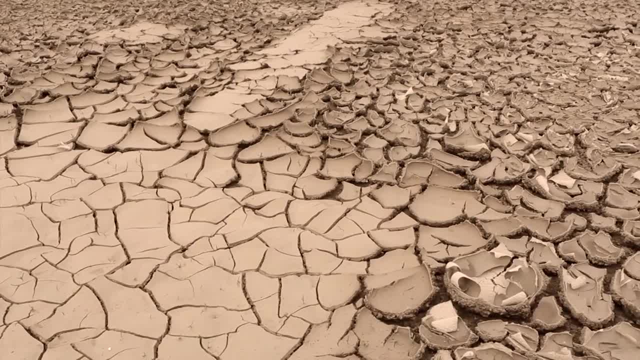 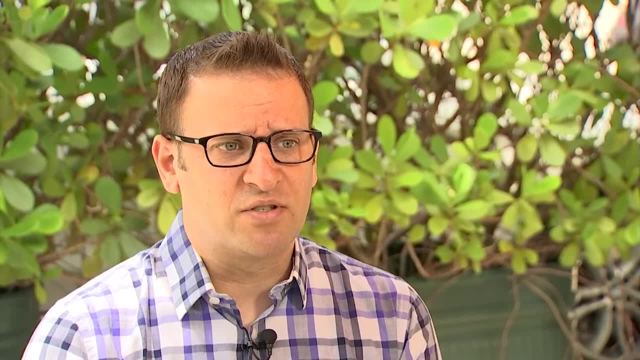 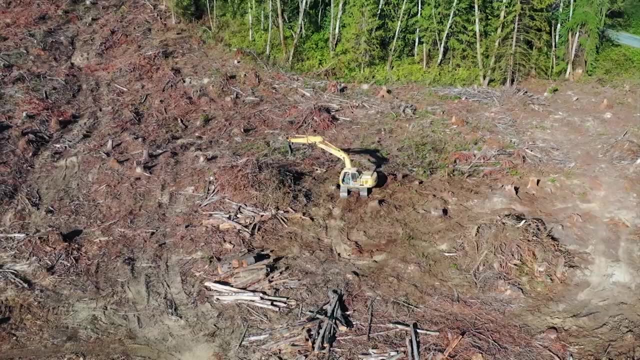 Climate change causes an increasing number of droughts and prolonged dry seasons. It also, during rainy seasons, creates precipitation to often come in more condensed bursts. These bursts make it more difficult for the land to absorb water. Water is also absorbed less by land that is deforested. 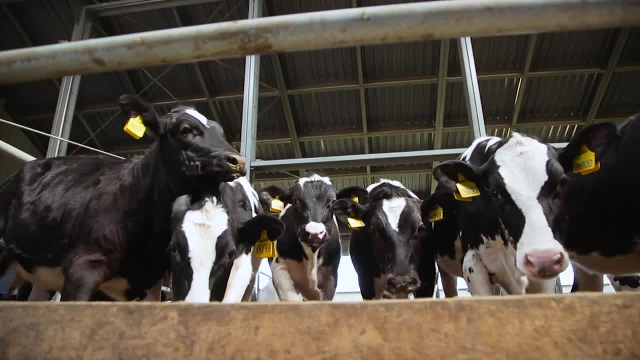 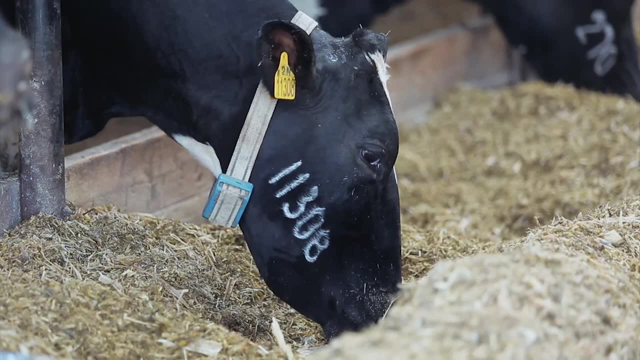 Forty percent of the world's land mass is occupied by livestock production. When forests are cut down to make room for animals, it's a triple whammy: Greenhouse gases are released into the atmosphere. there are less plants to take in carbon dioxide. 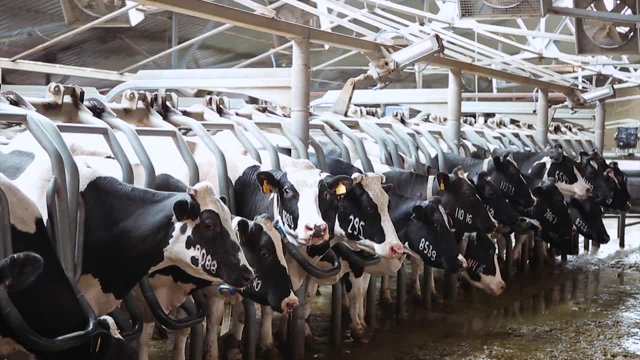 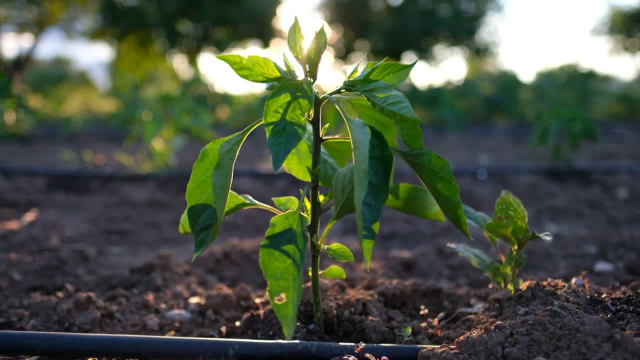 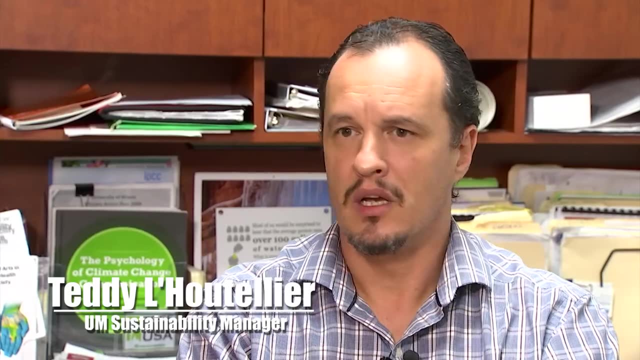 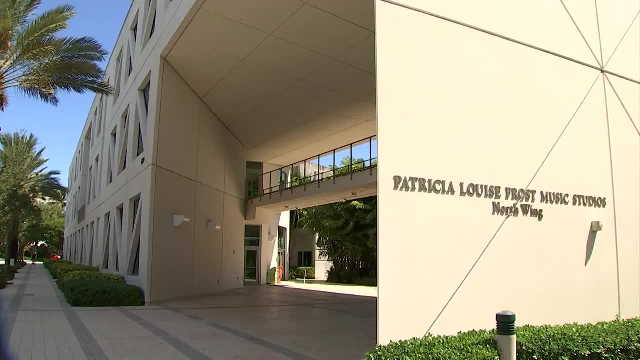 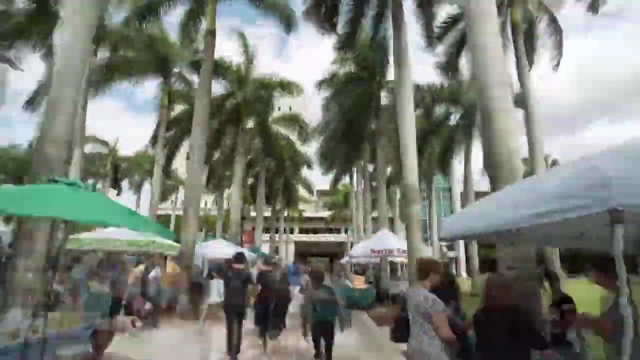 The University of Miami has pledged to reduce its carbon footprint. That means buildings that are LEED-certified and reduce emissions- energy, water and waste, But it also means educating students on their food choices. So trying to eat locally is definitely a way to lower the carbon footprint involved in those products that you eat. 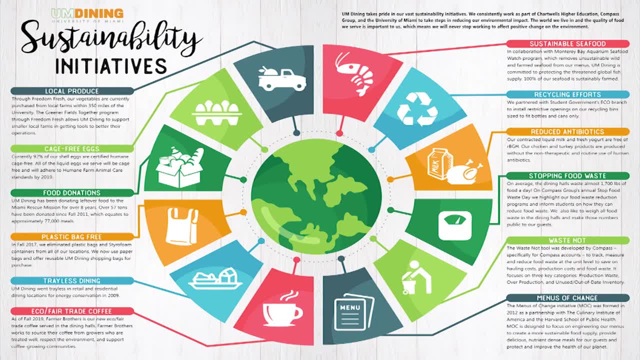 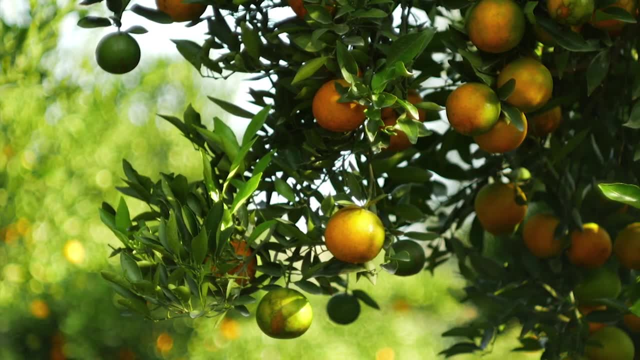 The reason is simple is if we farm and we grow food next to where we live, it's going to lower the carbon footprint. It's pretty simple to understand. The University buys local in-season food from distributors as much as possible and even has free food. 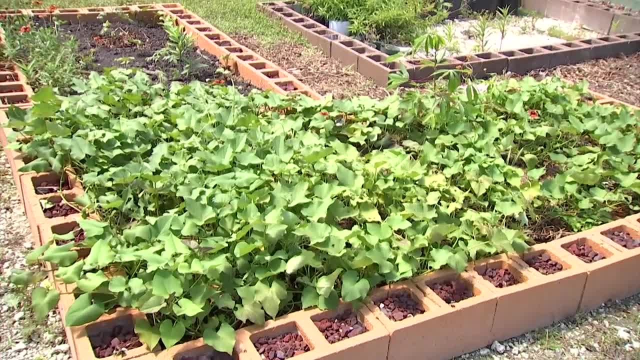 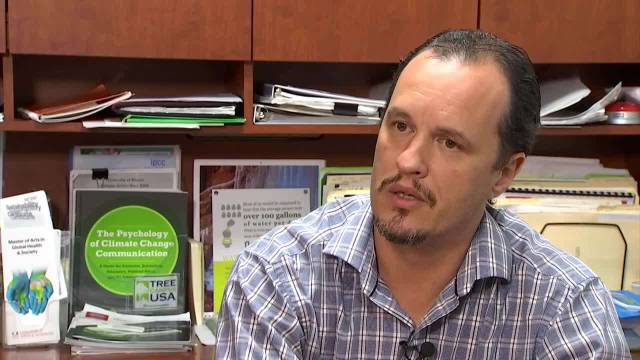 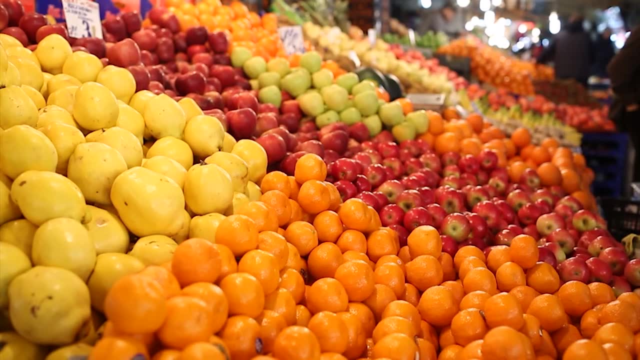 It has its own sustainable garden that will eventually serve students. It's not just about where the food is grown, but what type of food is available. When we promote dishes, we try to focus on the plant-based options. Plant-based options, otherwise known as vegan options, have proven health benefits. 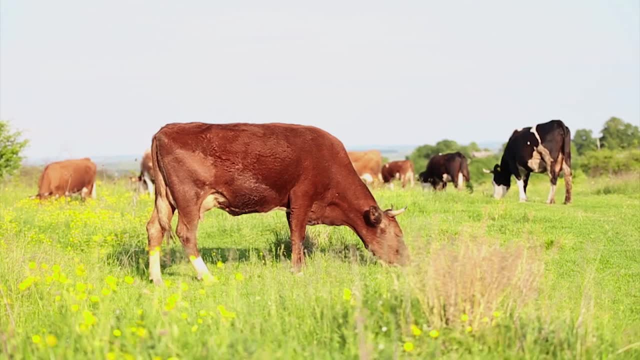 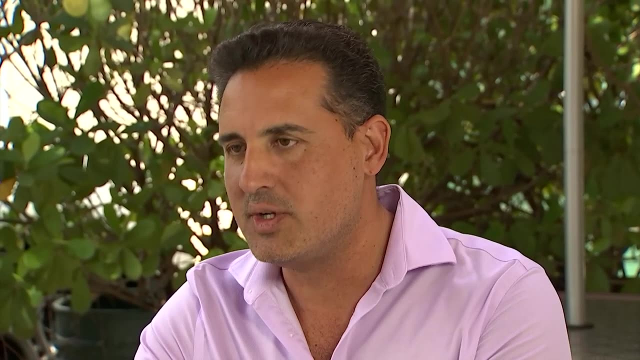 But veganism at its core is about animal ethics. I knew nothing about environmental issues until I became vegan. The movement brought me to climate and environmental issues: Climate and environmental understandings of what's happening in the world that I wasn't aware of before. 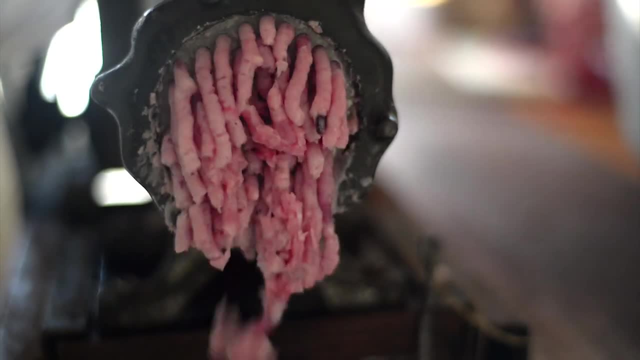 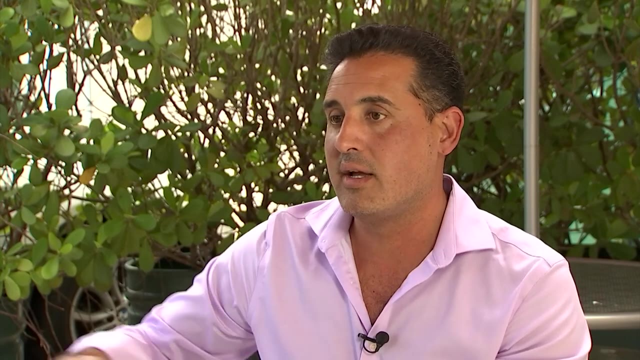 And to those who say we need to eat meat to get enough protein: We're basically getting the nutrients from the earth that we need to sustain ourselves through the animals. So they're the middleman. We can go straight to the proteins, straight to the nutrients. 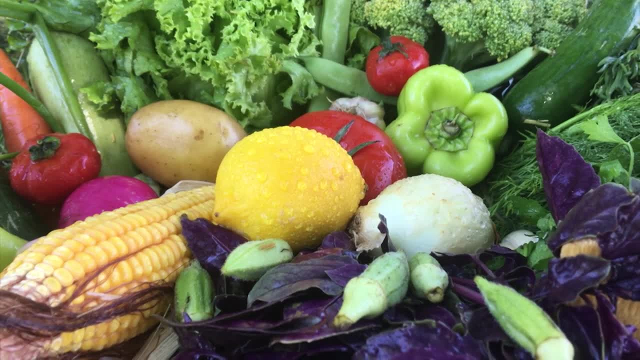 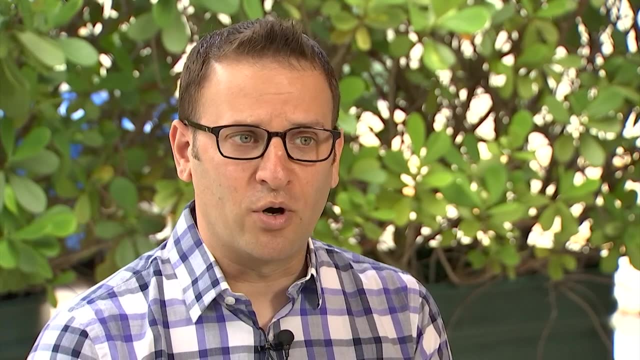 The message to get out to people is not necessarily everybody needs to become a vegetarian or a vegan overnight, but that small changes in the diet, like doing a Meatless Mondays program or just swapping out some beef for chicken, pork, turkey fish, things like that. 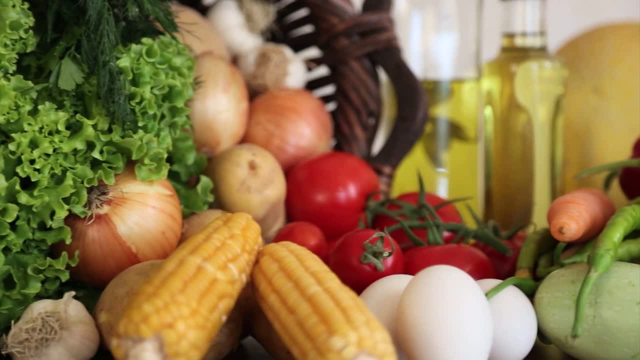 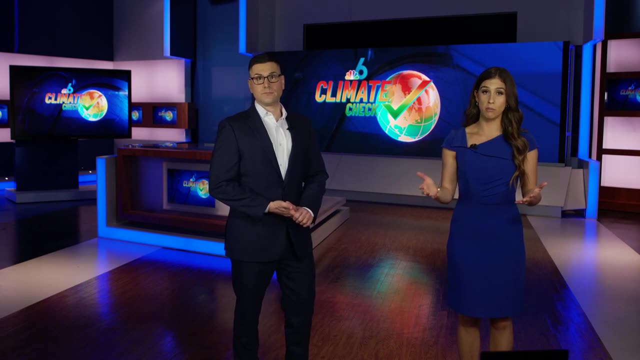 can actually make a measurable contribution to reducing emissions. Foods that are produced locally, like at UM, also cut down on air and car miles, which in turn cuts down on emissions. Now for those of you thinking of adding vegan meals to your diet, but not sure where to start: 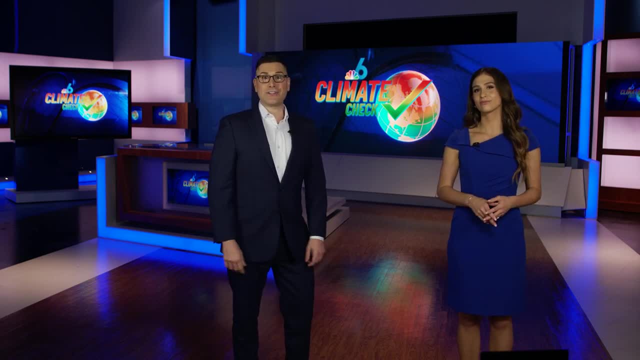 head over to my Facebook page, SteveMacNBC6.. I've posted a few of them. They're one of my favorite spots around South Florida. 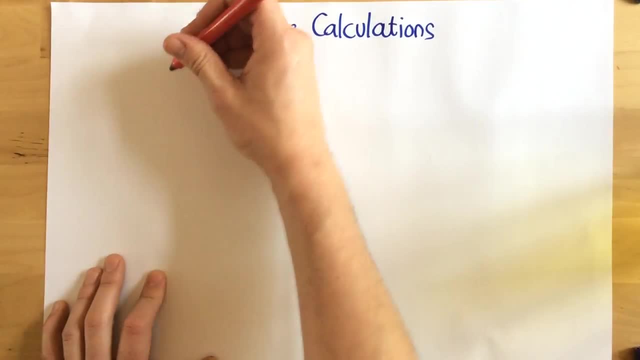 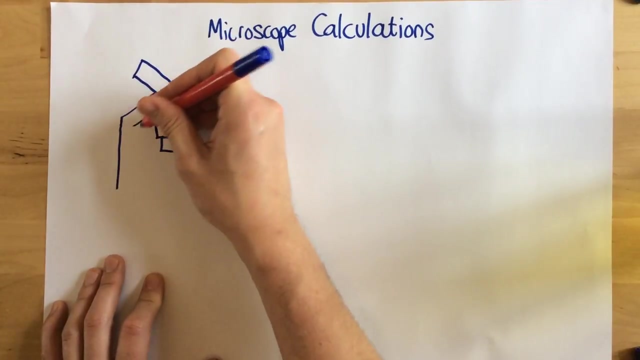 Okay, today I'm going to talk to you about microscope calculations, because there's two different types of calculation that we need to do when it comes to thinking about microscopes. So, to begin with, I'm just going to draw a diagram of a microscope. So, as a quick recap, 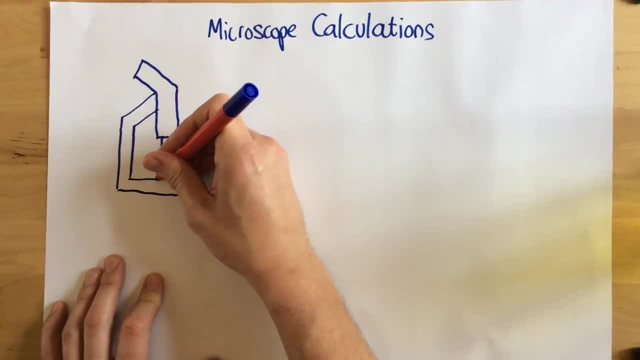 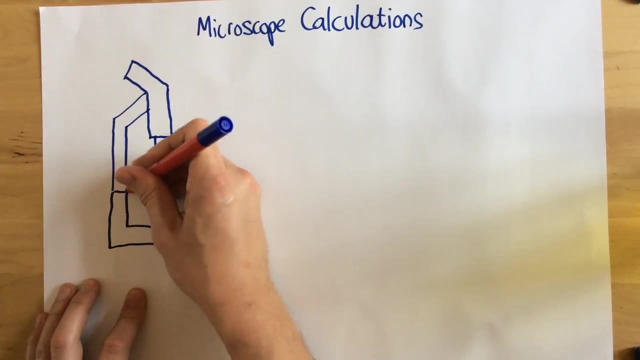 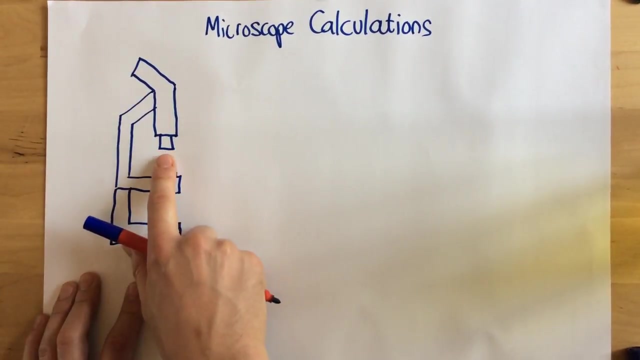 a microscope is a piece of equipment that we can use that magnifies an image. Now, the reason why we want to magnify something is if it's too small to see with the naked eye, for example cells. So we look down here the eyepiece lens and this is the objective lens. So we've got 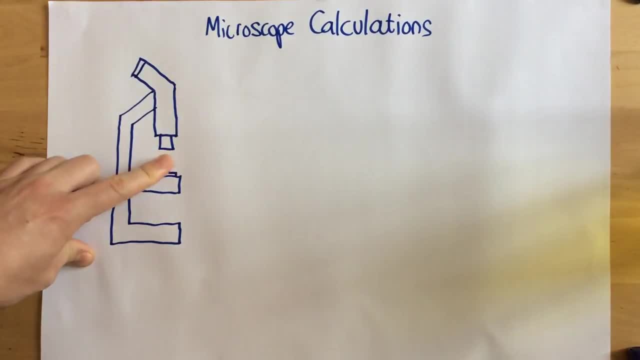 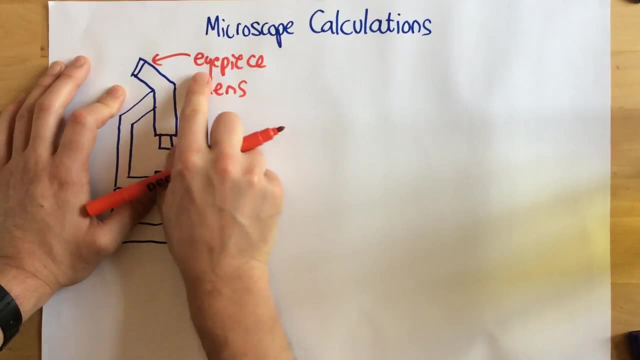 two different lenses which magnify the image. So first of all, here is the eyepiece lens, the bit that you look down. We know that this is this one because it goes next to your eye. so let's say, this one has a magnification of 10, which means it makes everything appear 10 times.